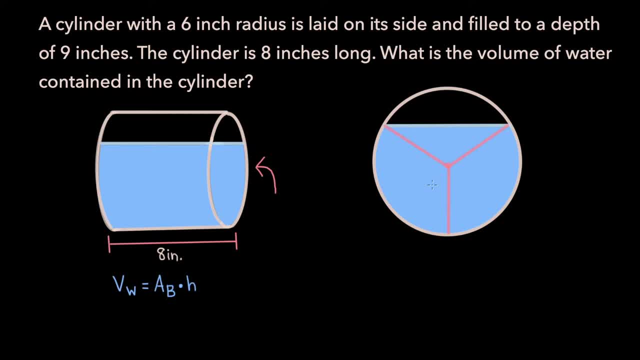 Both of which are shapes that we know to calculate the area of. Now, if we label the lengths we know, the problem tells us that the radius of the circle is 6 inches and that the height of the water, which is this height right here, is 9 inches. 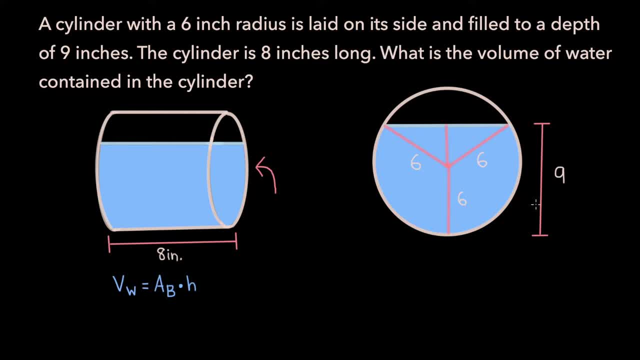 And this means that the height of our triangle is 9 minus 6, or 3 inches. These two angles must be 90 degrees, and notice that one of the legs in each of these right triangles that we formed is half the length of the hypotenuse, which is a hint that these two triangles are 30-60-90 triangles. 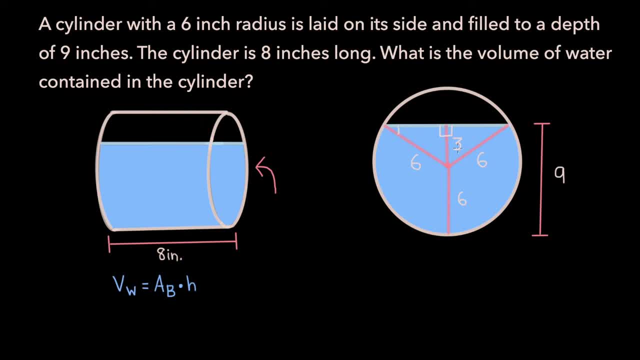 In a 30-60-90 triangle, the angle that is opposite the side, that is, half the length of the hypotenuse, is 30 degrees, which means that this remaining angle must be 60 degrees. And if we use the Pythagorean theorem on each of these right triangles, we get that the length of the remaining side is the square root of 6 squared minus 3 squared. 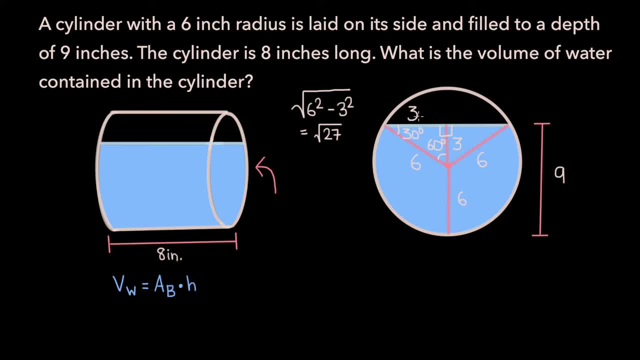 which is the square root of the hypotenuse. So we have a square root of 27,, which is 3 root 3.. And the same goes for this leg of this triangle as well, since both of these triangles are identical. Now, the area of just the triangle is 1 half base times height. 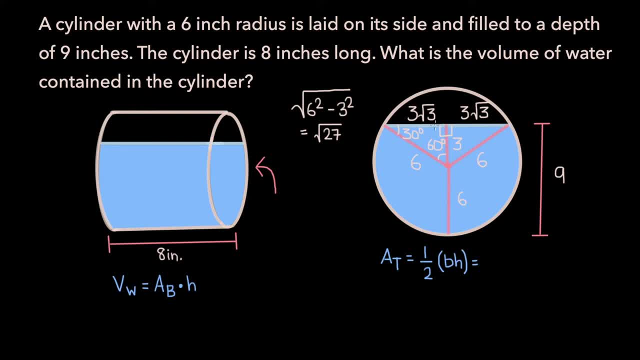 The length of the base is 3 root 3 plus 3 root 3, so 6 root 3.. And the height is just 3, so 1 half times 6 root 3.. Times 3,, which is 9 root 3.. 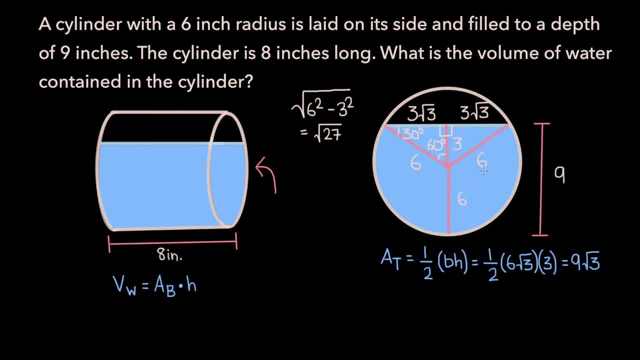 Now we need to find the area of the remaining portion of the base. Now, the technical term for this remaining portion is a sector, so I'll refer to it as that. from now on, This angle here must be 240 degrees, since this entire angle is 120.. 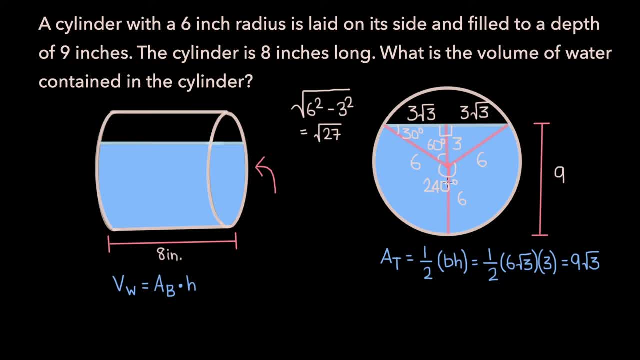 And what that means is that the sector must be 240 over 360, or 2 thirds of the entire circle, And so the area of the sector is 2 thirds pi r squared, where r is equal to 6.. So 2 thirds times pi, times 6 squared, which is 36,, which is equal to 24 pi.